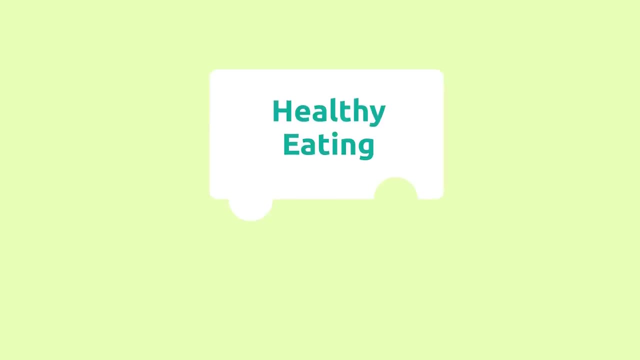 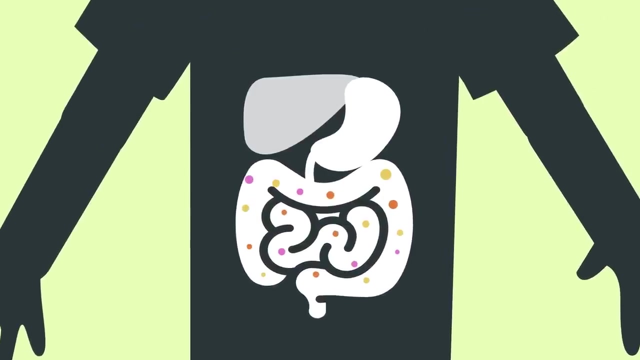 eat healthy. Healthy eating should be complete, including foods that contain all nutrients, and balanced, That is to say, our intake of every nutrient should come in the right proportions. During the digestion process, nutrients in foods are absorbed in the intestines and from. 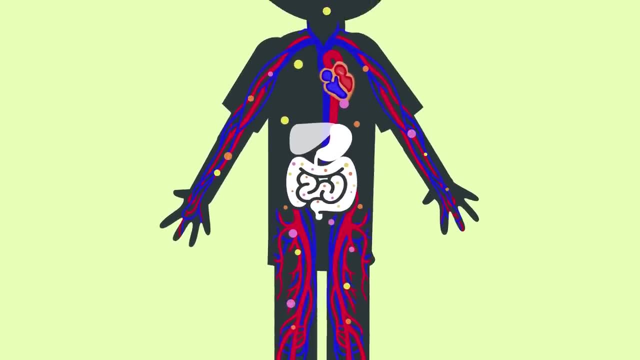 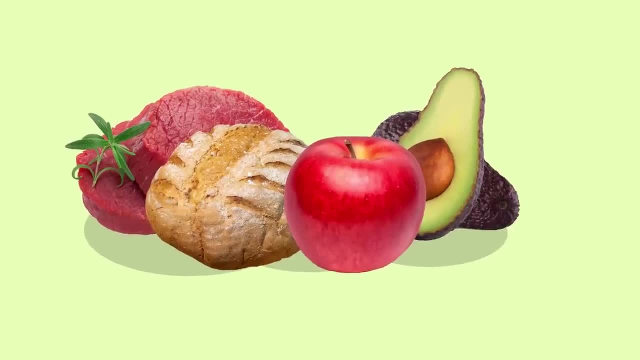 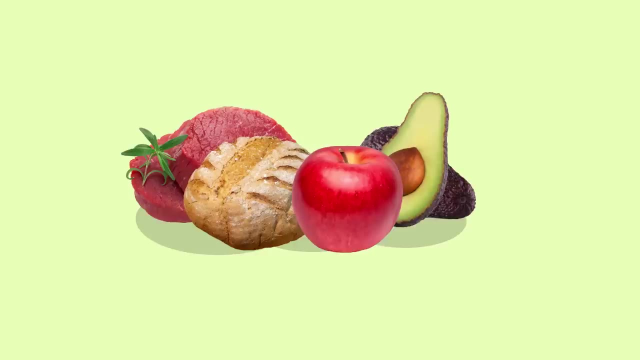 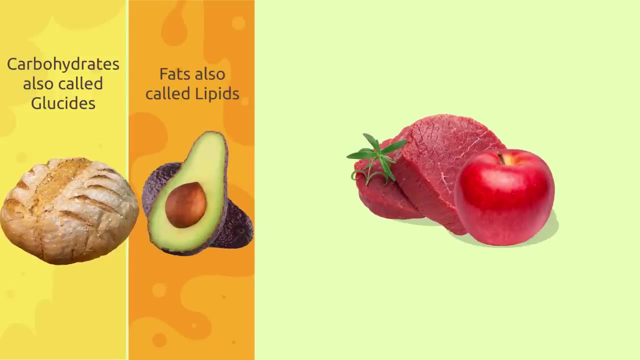 there they are distributed all over our body through the circulatory system. Food Nutrients. We could group food sources in many different ways. One way of doing that is by looking at the nutrients they provide. These nutrients are Carbohydrates, also called glucides, Fats, also called lipids. 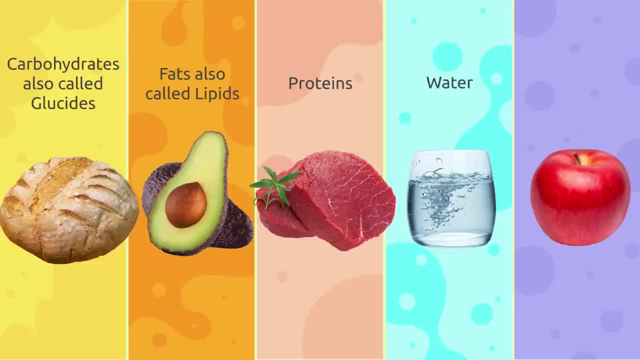 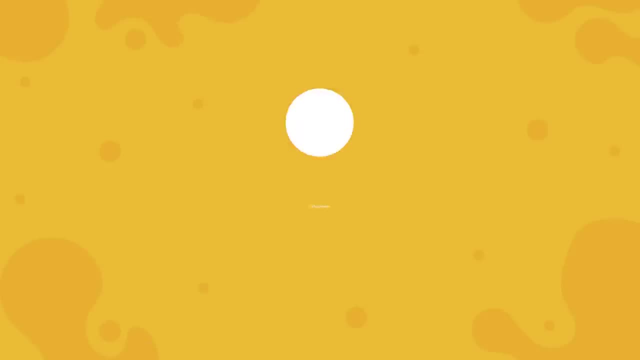 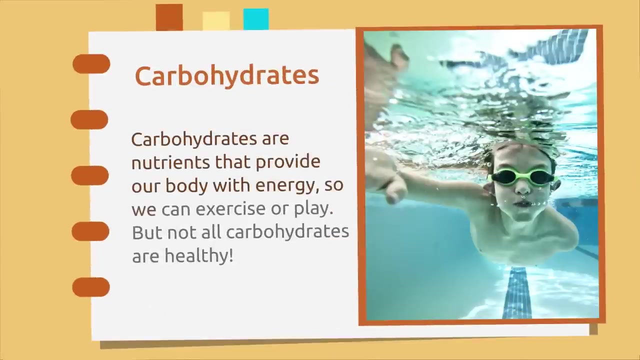 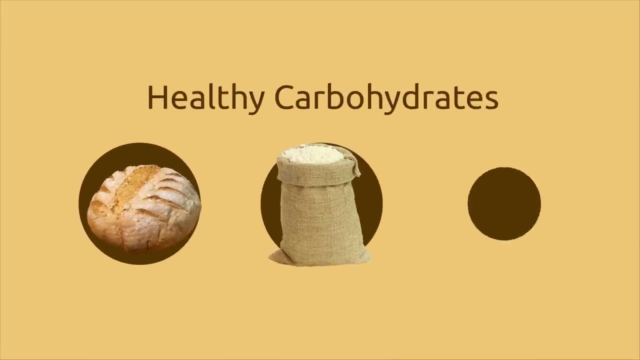 Proteins, Water, Vitamins and mineral salts. Would you like to learn more about them? Carbohydrates: Carbohydrates are nutrients that provide our body with energy so we can exercise or play, But not all carbohydrates are healthy. Bread, rice or pasta are healthy high-carb foods. 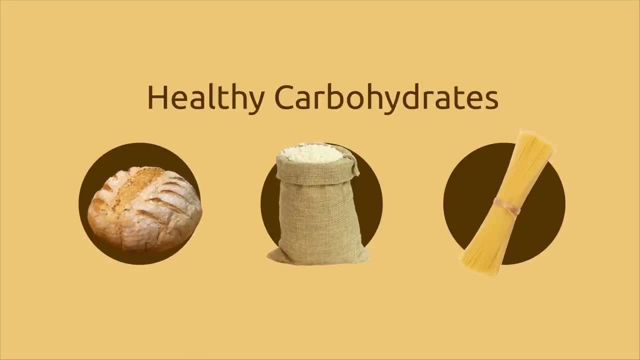 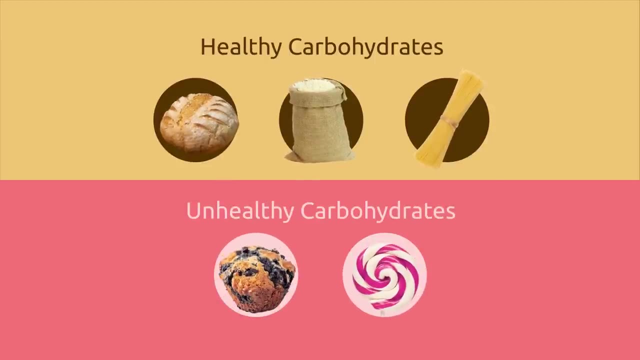 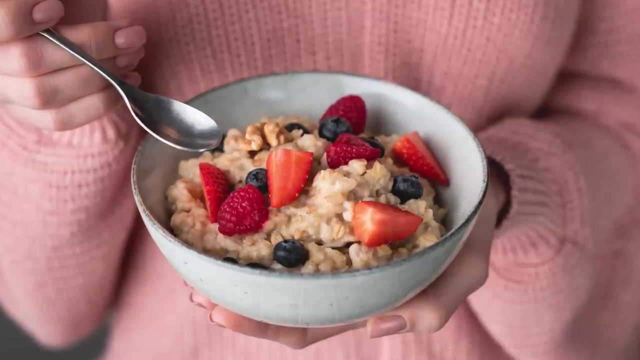 There are high-carb foods, also called foods high in glucides, that are not good for our health. An example would be sweets like pastries or candy. Eating fruit is a healthy way to include glucides or carbohydrates in your diet. Besides, fruits provide us with vitamins too. 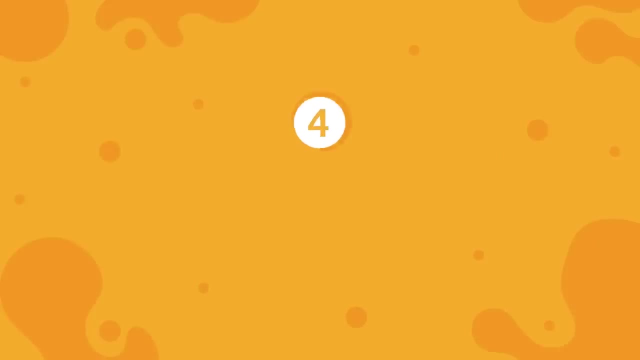 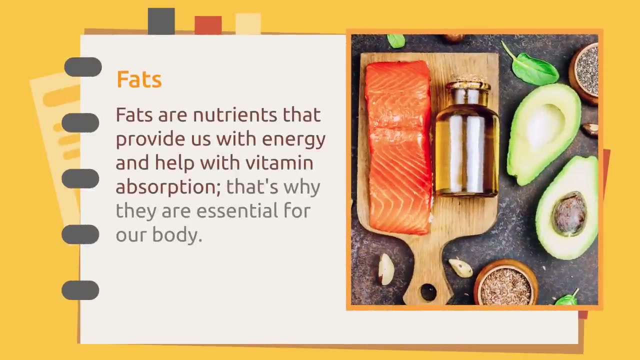 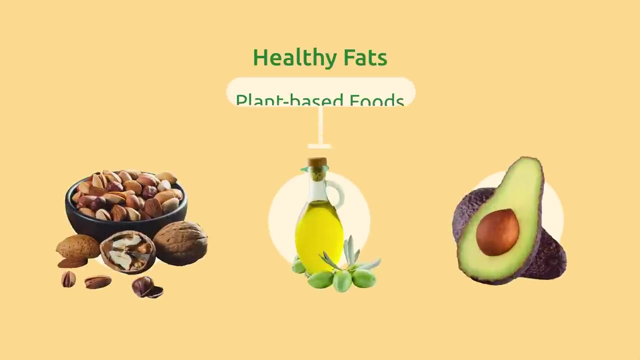 Fats, Fats or nutrients that provide us with energy and help with vitamin absorption. That's why they are essential for our body. Nuts, avocados or olive oil are high-carb fats. Avocados or olive oil are high-fat foods. 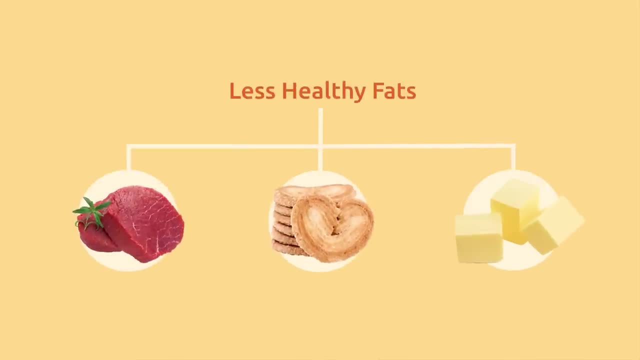 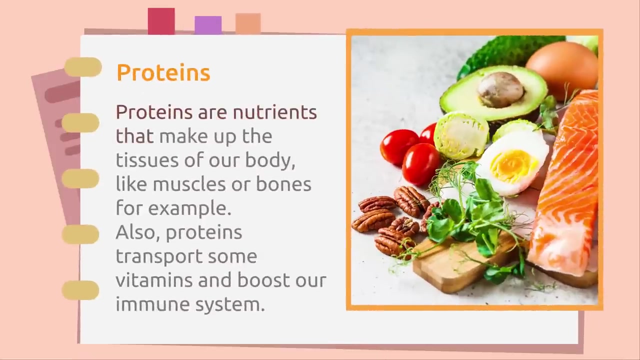 Other foods, like meat or butter, are also high in fats. Eating too much of them may be harmful to your health. Eating healthy is not about adding many high-fat foods to your diet- Proteins- Proteins are nutrients that make up the tissues of our body, like muscles or bones, for example. 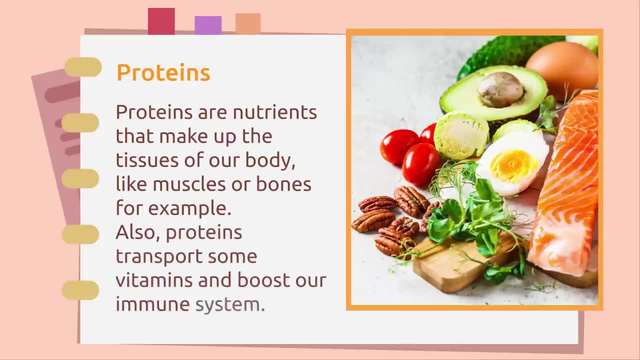 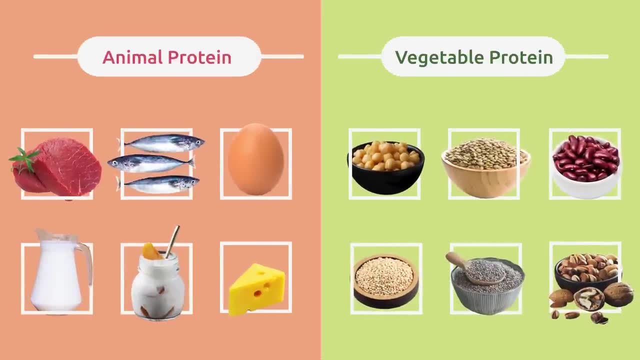 Also proteins transport some vitamins and boost our immune system. Animal proteins are found in food sources like meat, fish, eggs or dairy products. There are also vegetable proteins, like the ones found in legumes. Remember to combine both for a balanced diet. 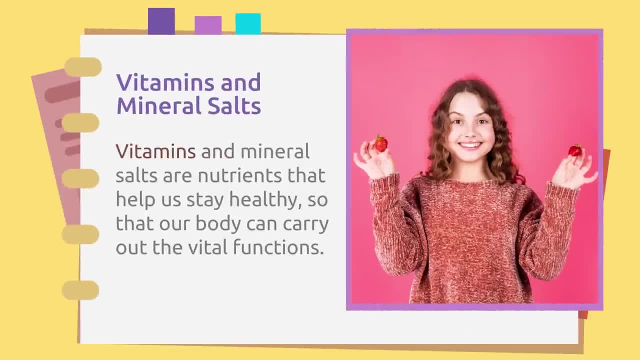 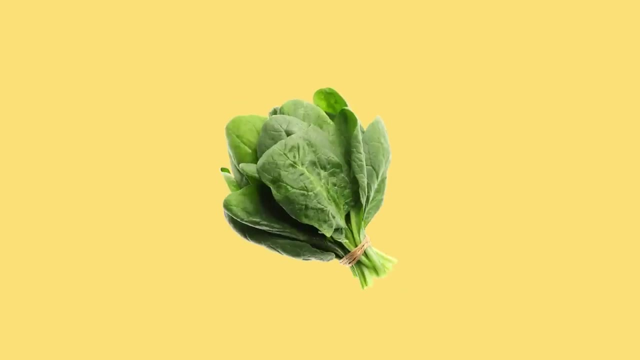 Vitamins and mineral salts. Vitamins and mineral salts are nutrients that help us stay healthy so that our body can carry out the vital functions of our body. Fruits like oranges, strawberries or bananas and leafy greens or vegetables like spinach, broccoli or carrots are packed with vitamins. 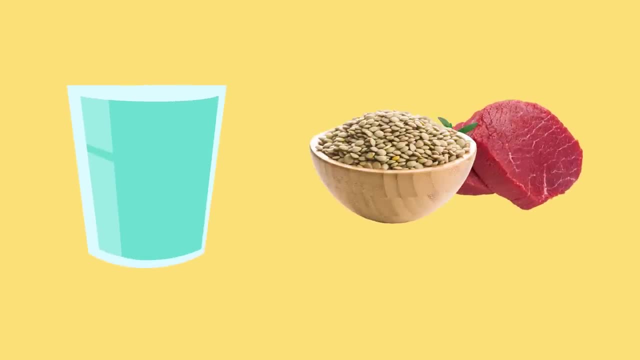 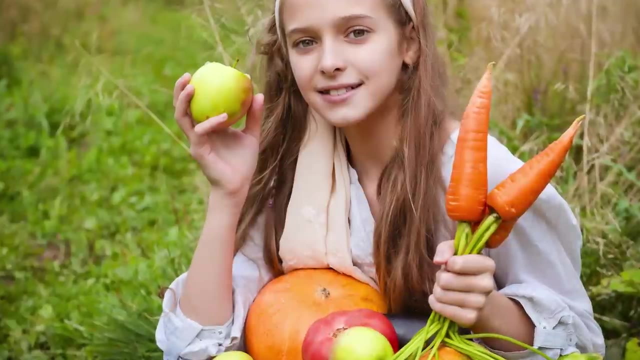 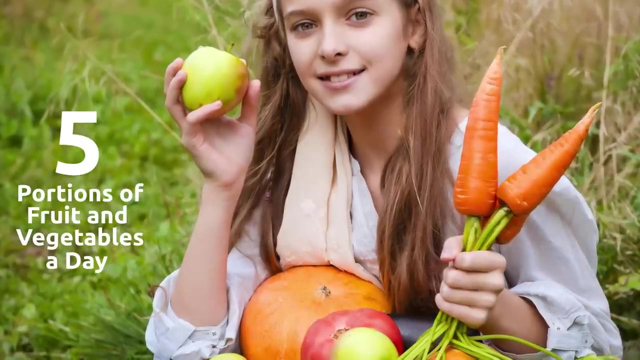 Minerals are found in the water in small amounts and in different types of food, like lentils or meat that contain iron. Did you know that in order for our body to get the vitamins it needs, it needs to be eating at least 5 portions of fruit and vegetables a day? 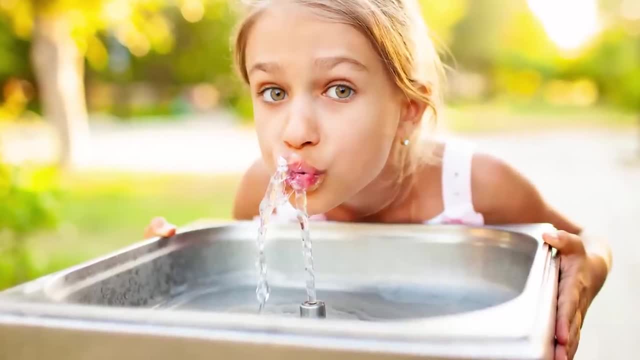 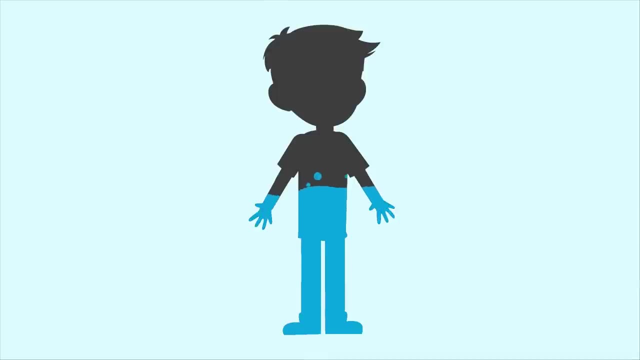 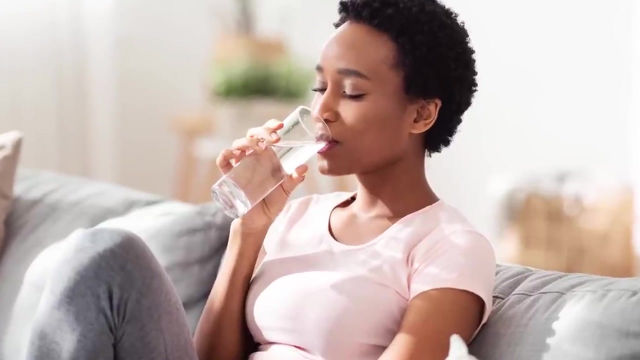 Water. Water is very important in order for us to stay hydrated. It is the most abundant substance in all living beings. Did you know that the majority of your body consists of water? That's why it is vital to drink water throughout the day, and drink even more when we do physical. 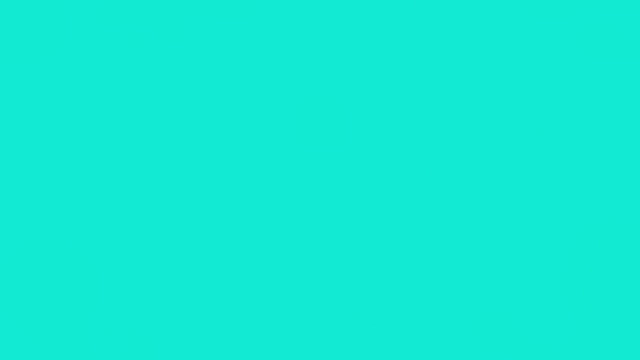 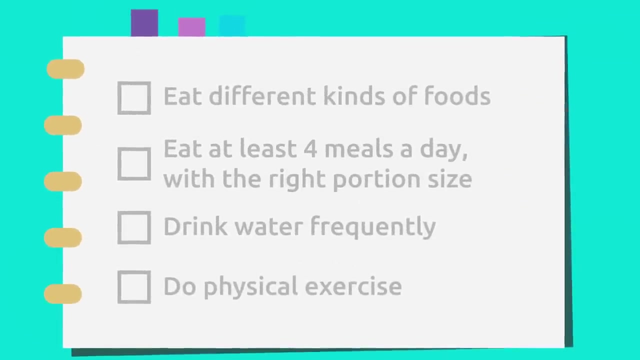 exercise or when it's hot Water is important for our body. We all lose weight after drinking water. That's why our body goes through a lot of health issues. So while we may lose weight, we should always make sure to fish on the right food to keep. 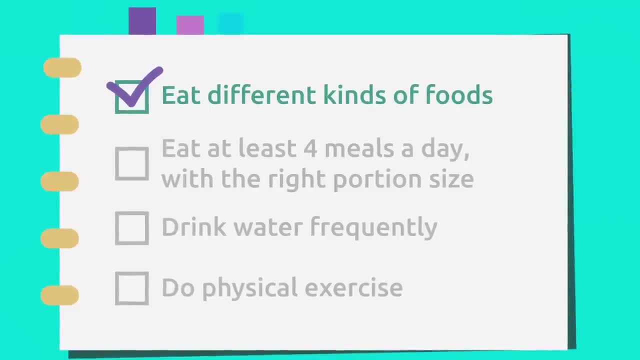 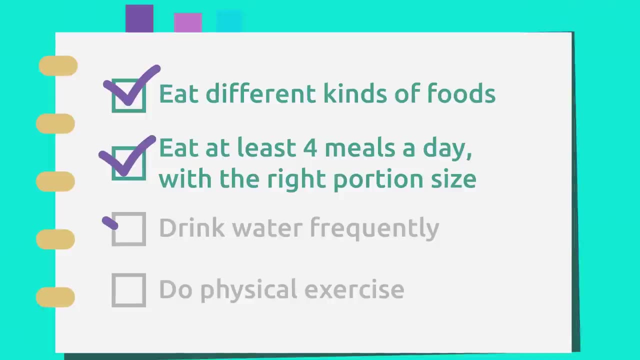 ourselves in shape so that we can recover from the upcoming health issues. If food can make your body full, you need a healthy diet. What are some good health tips? How to increase your Giraffe To have a healthy diet. we recommend to follow this advice. 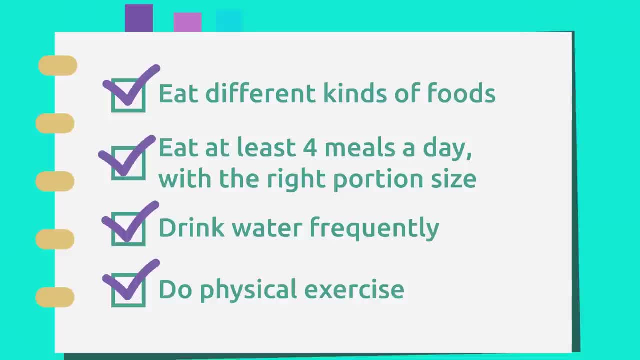 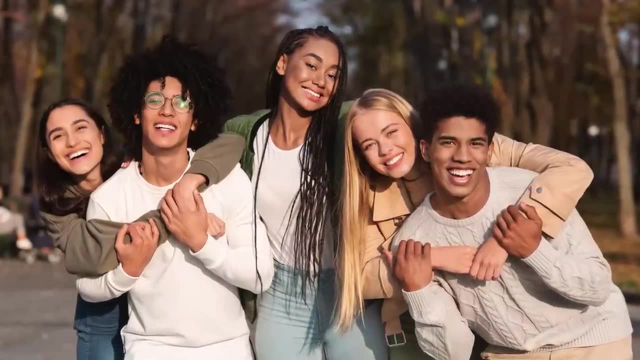 Eat different kinds of foods. that will provide you with all the nutrients you need. Eat 4 meals a day with proper portion size. Drink water frequently to stay hydrated. eaten. If you follow this advice, you'll be preventing diseases like obesity or diabetes.